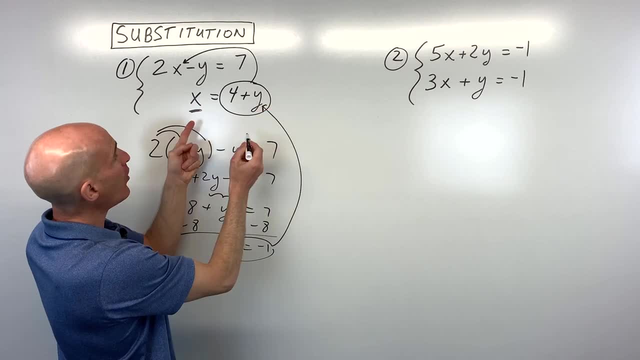 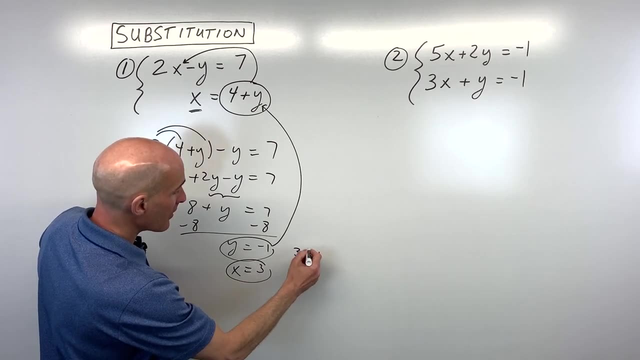 we already have x by itself, So let's go ahead and put negative 1 in for y. 4 plus negative 1 is 3.. So now we know x equals 3. And we can write this as a coordinate pair. 3 comma. 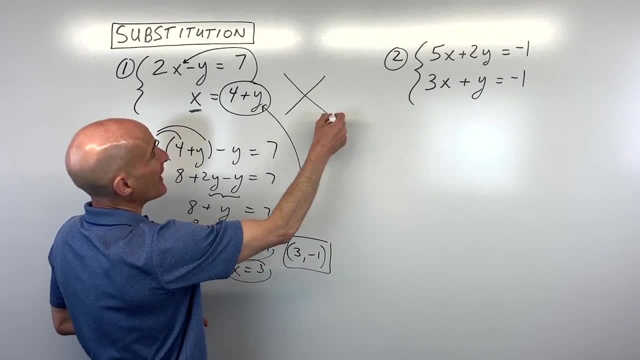 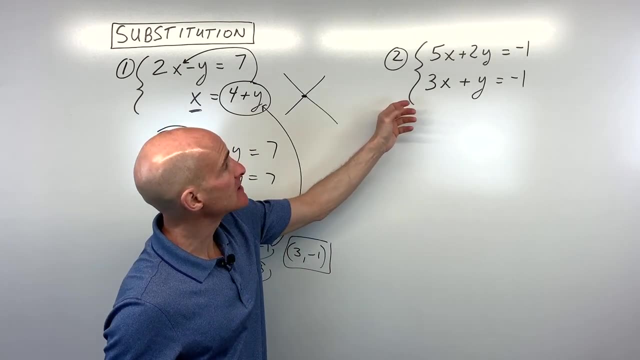 negative 1.. So what this means is, if we were to graph these two lines, the point where they intersect is going to be 3, negative 1.. Okay, example number 2 is a little bit more challenging, because it wasn't like this one, where we already knew what one of the 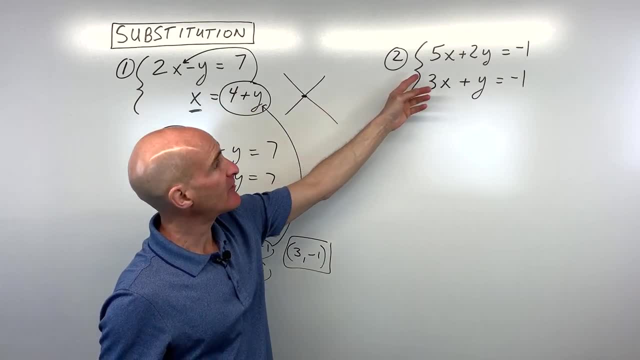 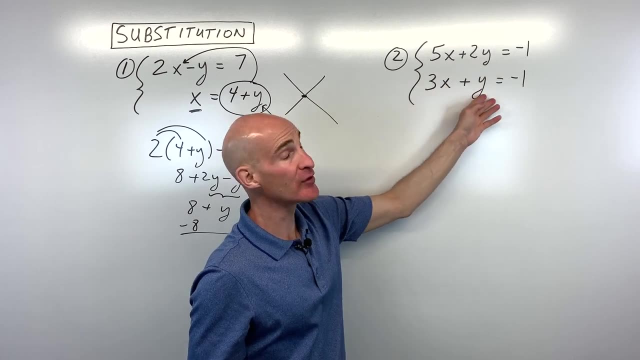 variables equaled. We have x equals. Over here you have to decide: should I solve for this x and find out what x equals, Or should I solve for this y and find out what y equals, Or this x or this y. 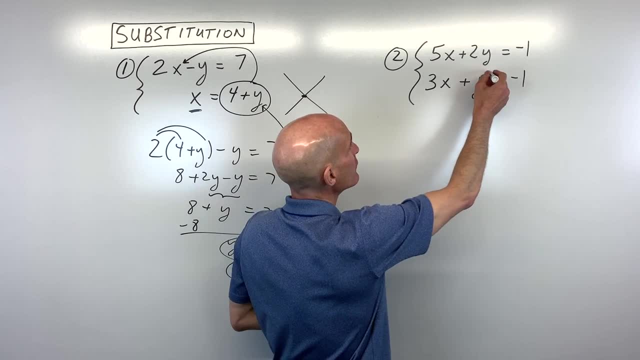 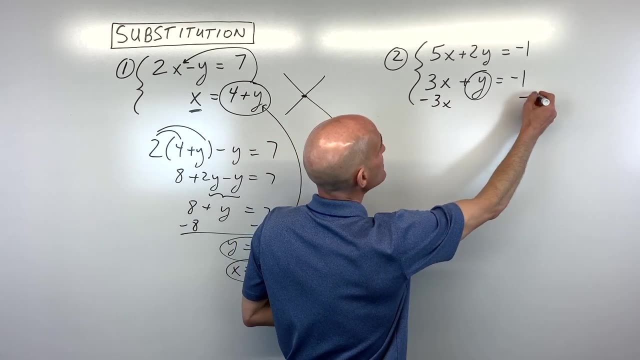 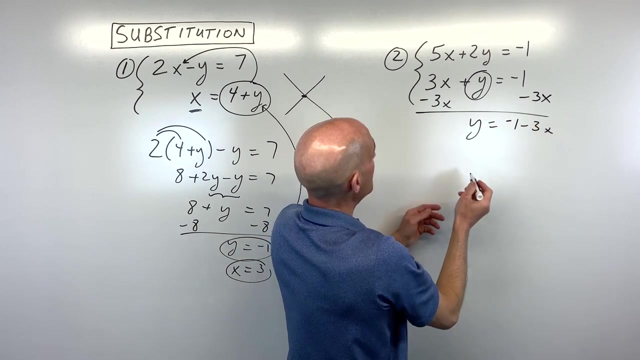 Well, in this particular problem it's going to be easier to solve for this y, because you only have one y, so you won't have to divide. So all we're going to do is we're just going to subtract 3x from both sides of the equation. So now we get y equals negative 1 minus 3x. 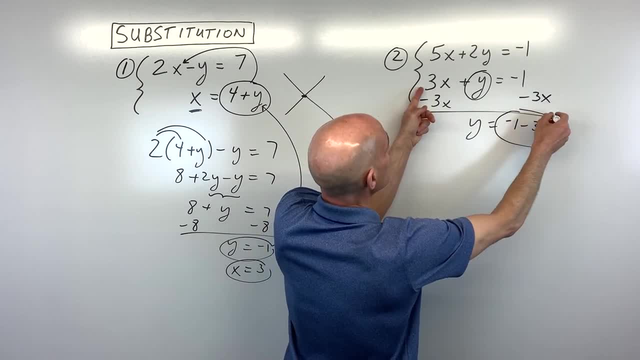 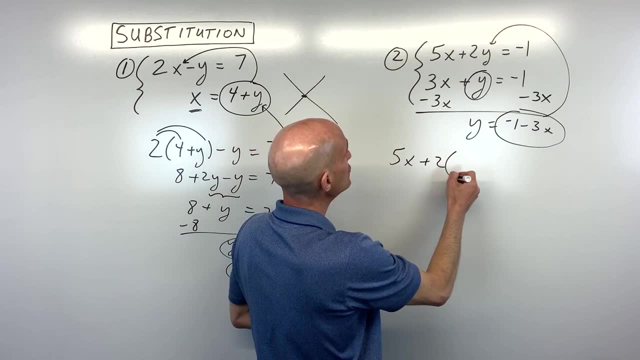 and so that was for the second equation. So now we know what y equals, Let's go ahead and put it in for y in the equation that we haven't used yet, the first equation. So we have 5x plus 2 times Now. instead of y, I'm going to put 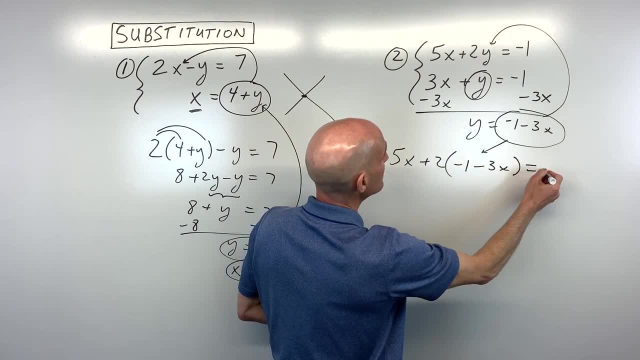 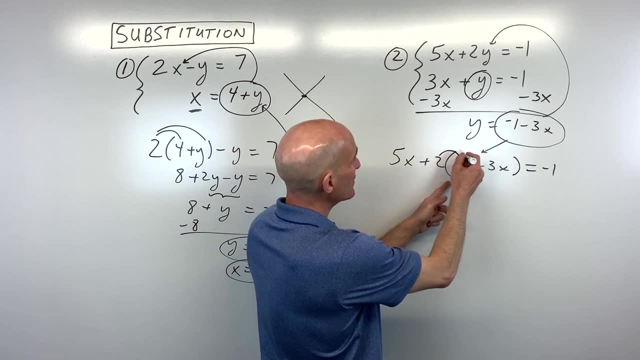 Well, y equals negative 1 minus 3x equals negative 1.. And again, remember, when you do that substitution, put it in parentheses so you can treat it as a group. So now what we want to do is we want to distribute the 2, and that's going to give us negative 2 minus 6x. 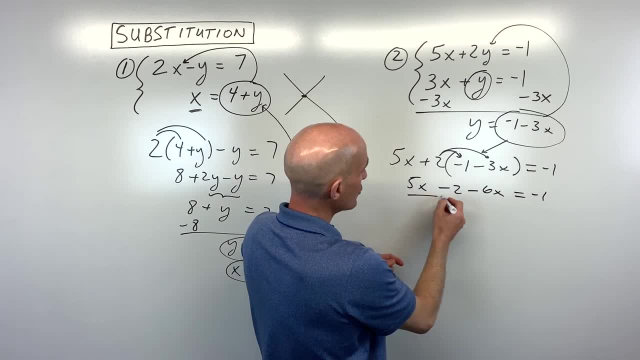 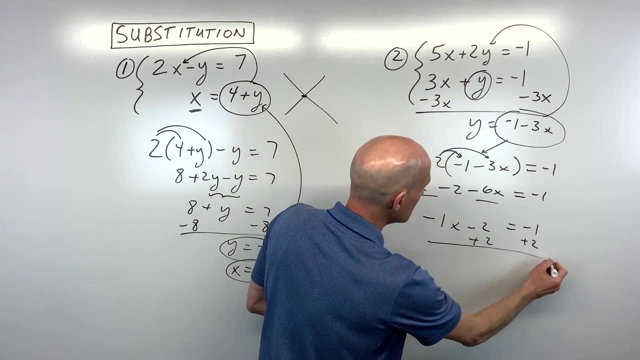 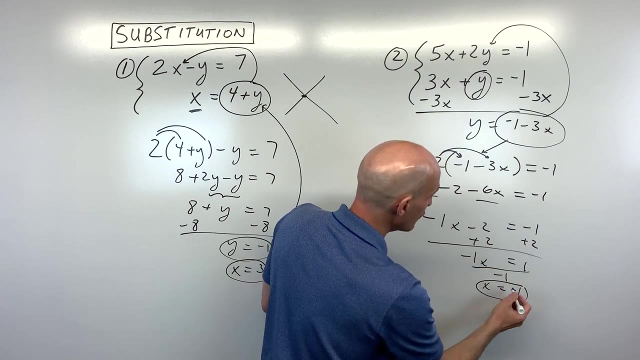 Bring down the 5x. Combine like terms 5x and negative. 6x is negative 1x. Add 2 to both sides And we get negative. 1x is equal to 1.. Divide both sides by negative 1, and you can see x equals negative 1.. 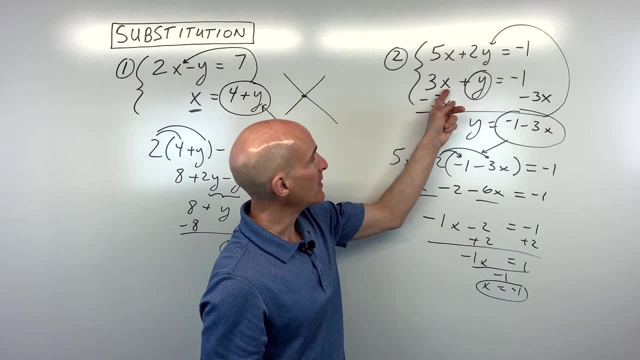 Now, if we take negative 1, we can put it back in for x here or here or here. I'm going to do this one because we already have y by itself, So we're going to put negative 1 right back in there. 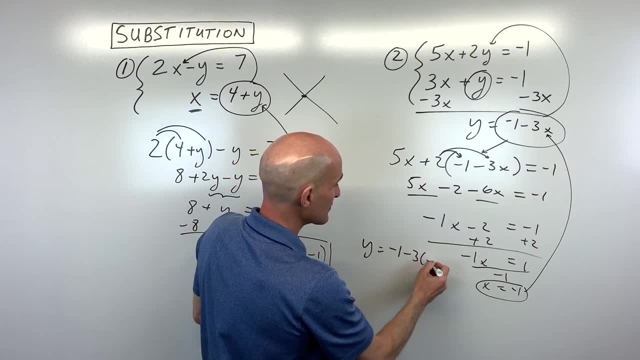 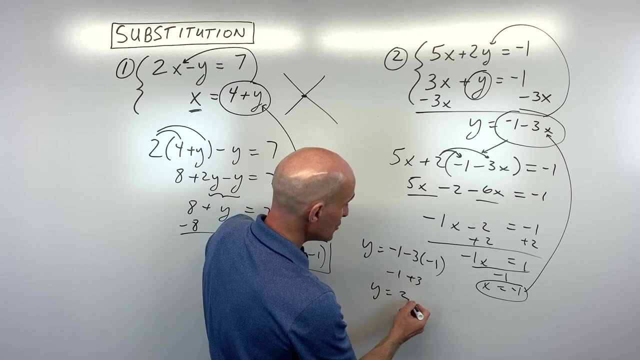 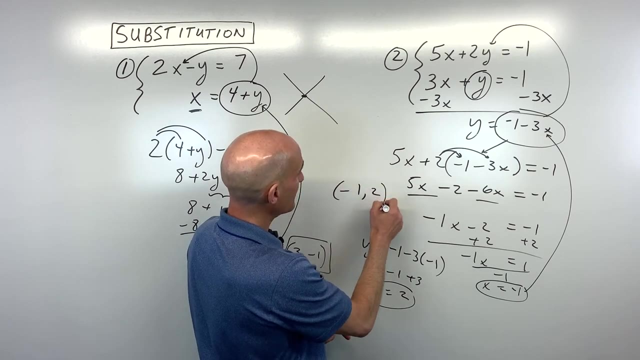 So that's going to give us: y equals negative 1 minus 3 times negative 1.. Negative 3 times negative, 1 is positive 3.. And so then y is equal to 2x, And so when we write our final answer, we want to write it as a coordinate pair: x comma y, or in this case, negative 1 comma 2.. 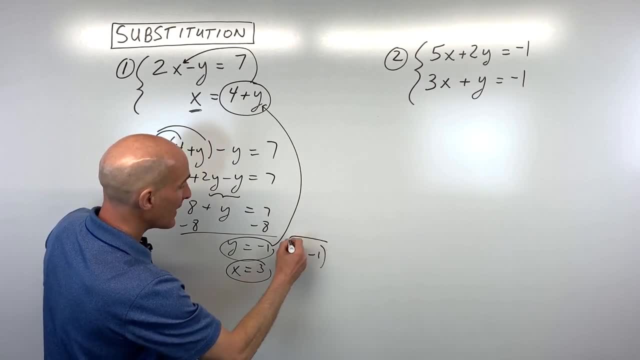 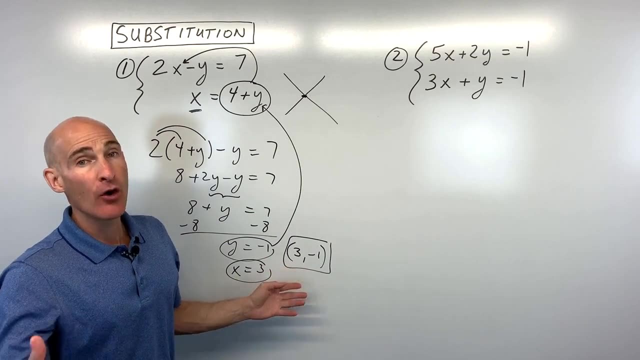 and we can write this as a coordinate pair: 3 comma negative 1.. So what this means is, if we were to graph these two lines, the point where they intersect is going to be 3 negative 1.. Okay, example number two is a little bit more challenging because it wasn't like this one. 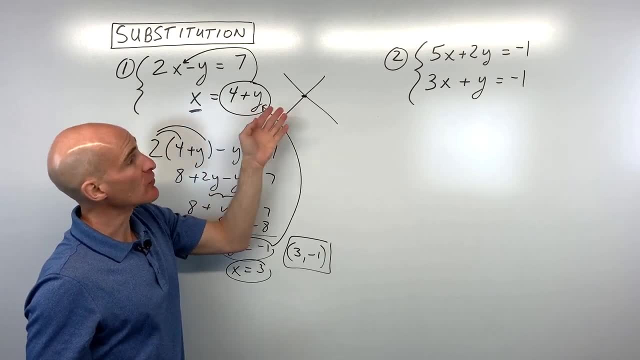 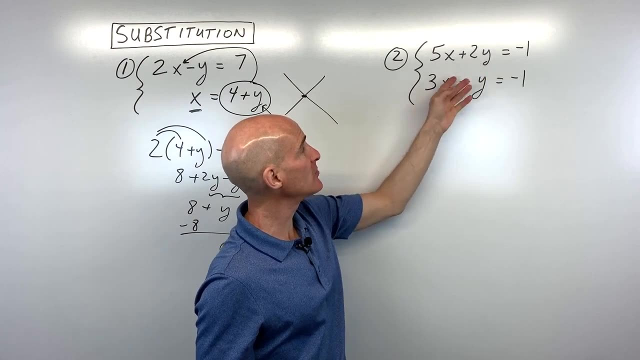 where we already knew what one of the variables equaled. We have x equals. Over here you have to decide: should I solve for this x and find out what x equals, or should I solve for this y and find out what y equals, or this x or this y? Well, in this particular problem it's going to be. 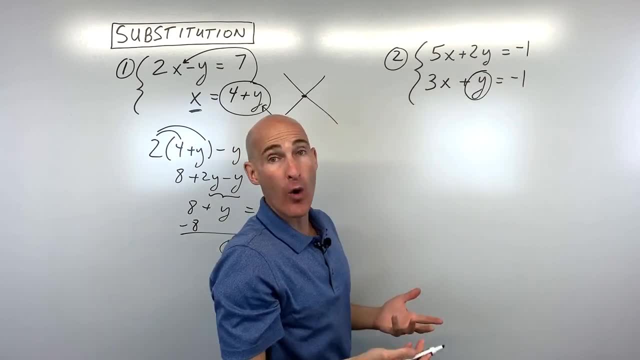 easy to solve for this y and find out what y equals, or this x or this y. It's going to be easier to solve for this y because you only have one y, so you won't have to divide. So all we're going to do is we're just going to subtract 3x from both sides of the 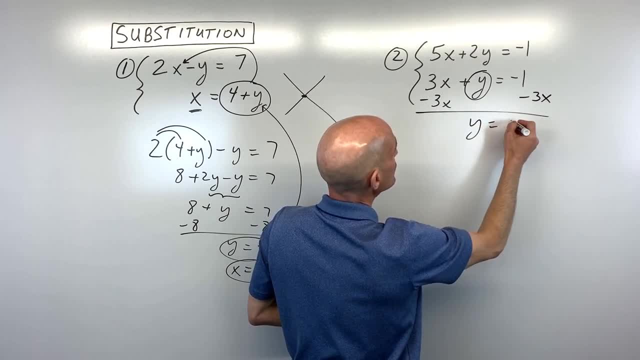 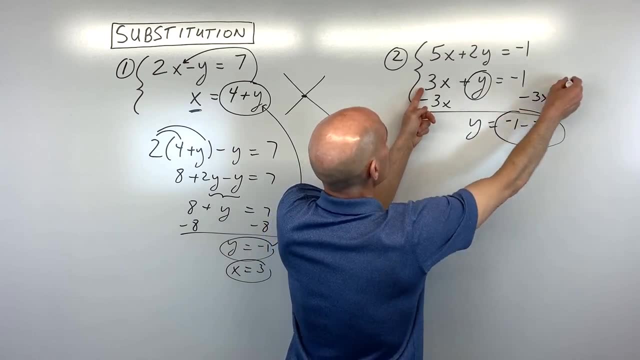 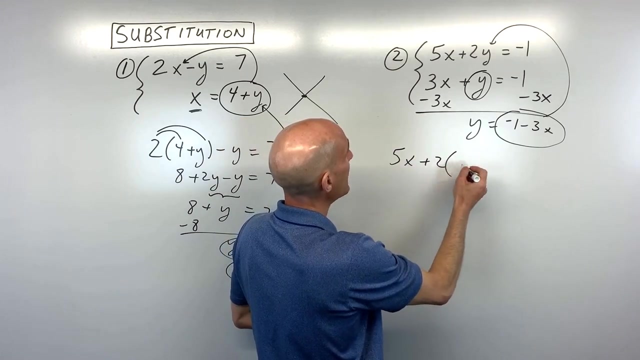 equation. So now we get: y equals negative 1 minus 3x, and so that was for the second equation. So now we know what y equals. Let's go ahead and put it in for y in the equation that we haven't used yet, The first equation. So we have 5x plus 2 times. Now instead of y I'm going to put what y. 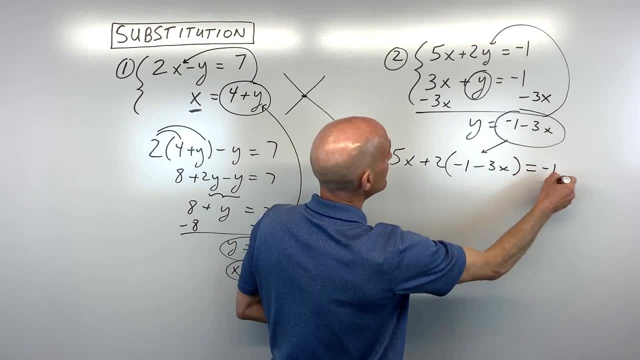 equals Negative 1 minus 3x. So now we have 5x plus 2 times. Now, instead of y I'm going to put 3x equals negative 1.. And again, remember, when you do that substitution, put it in parentheses. so 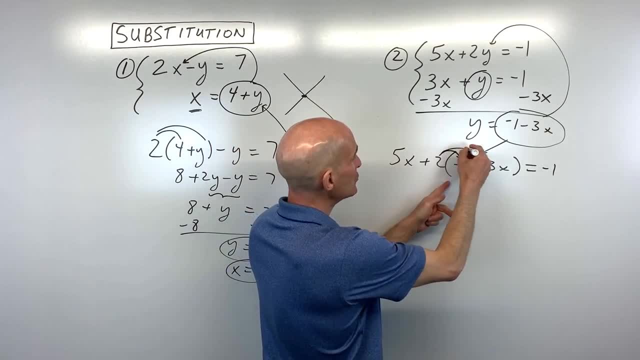 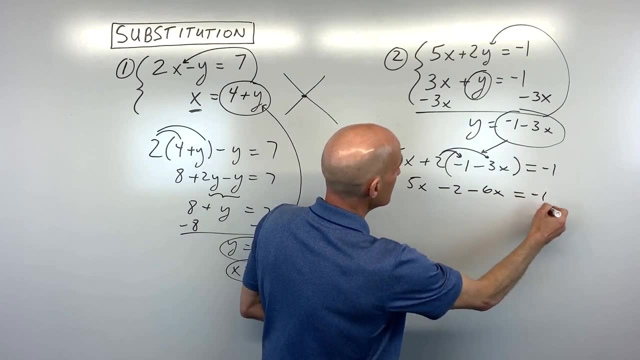 you can treat it as a group. So now what we want to do is we want to distribute the 2, and that's going to give us negative 2 minus 6x. Bring down the 5x, Combine like terms 5x and negative 6x. 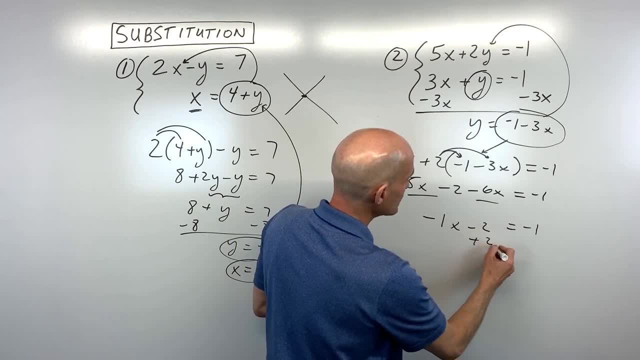 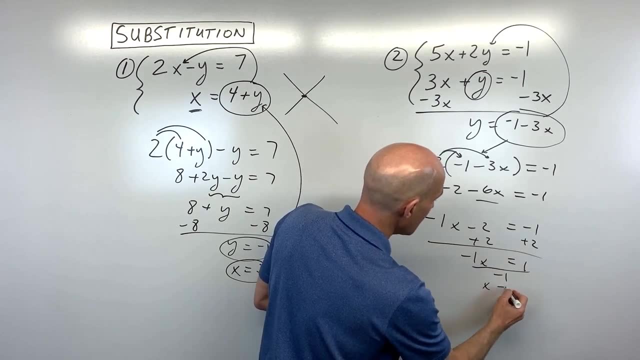 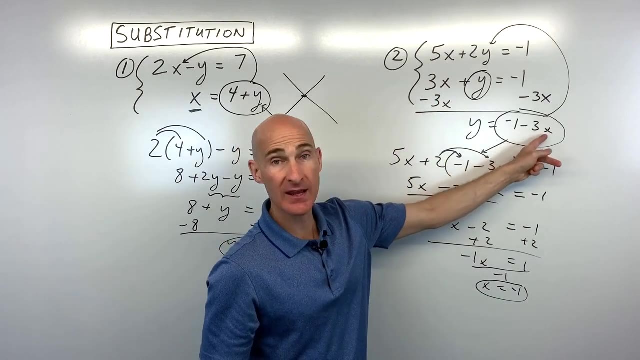 is negative 1x. Add 2 to both sides and we get negative. 1x is equal to 1.. Divide both sides by negative 1 and you can see: x equals negative 1.. Now, if we take negative 1, we can put it back in for x. here or here or here I'm. 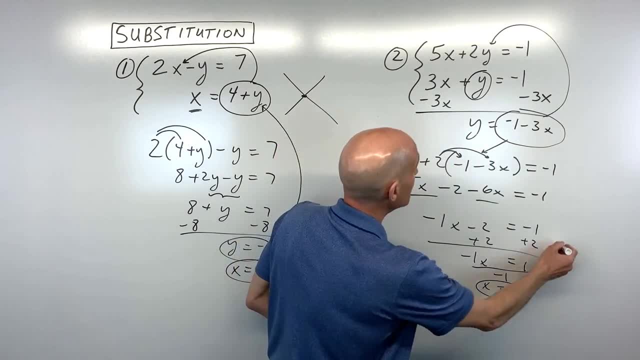 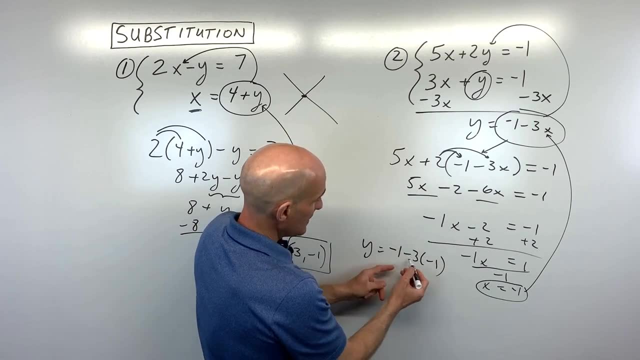 going to do this one, because we already have y by itself. So we're going to put negative 1 right back in there. So that's going to give us y equals negative 1 minus 3 times negative 1.. Negative 3 times negative 1 is positive 3.. And so then y is equal to 2.. And so when we write our final answer, 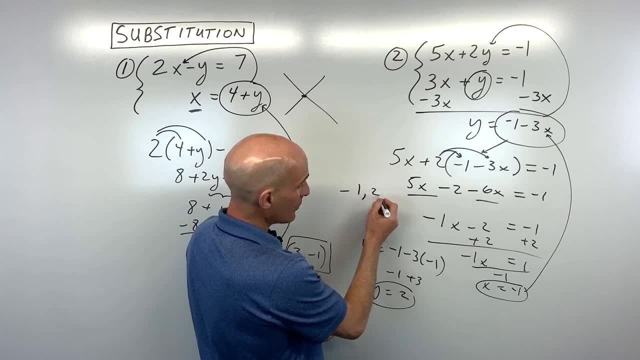 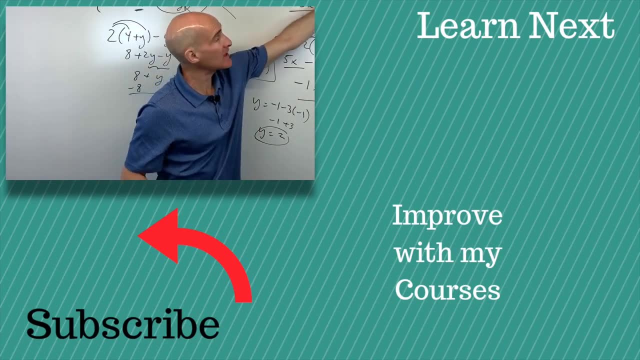 we want to write it as a coordinate pair: x comma y, or in this case, negative 1 comma 2.. Now, if you want to check your answer, you can always put negative 1 and 2 in for x and y and see if it equals negative 1.. Same thing here. Make sure it equals this value. Make sure it makes. 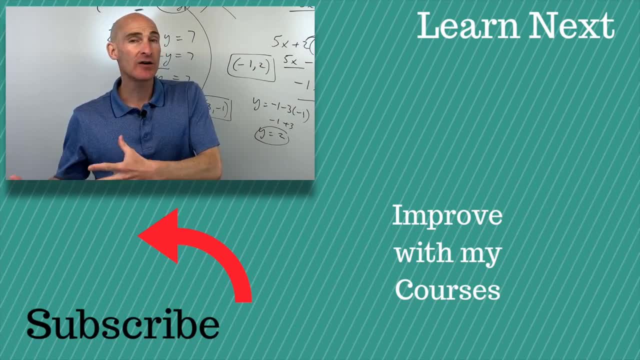 both equations true. Now the next thing you want to learn is how to solve systems using the elimination method. Follow me over to that video right there where we dive into elimination. 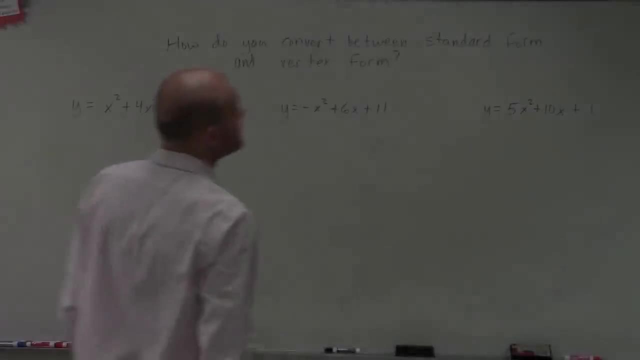 Welcome. So I have a whole little playlist on how to convert from standard form to vertex form, but I figured I'd just do one little video just so you have an idea, in case you come across some problems where you have to being able to solve or graph, you have to be able to convert from. 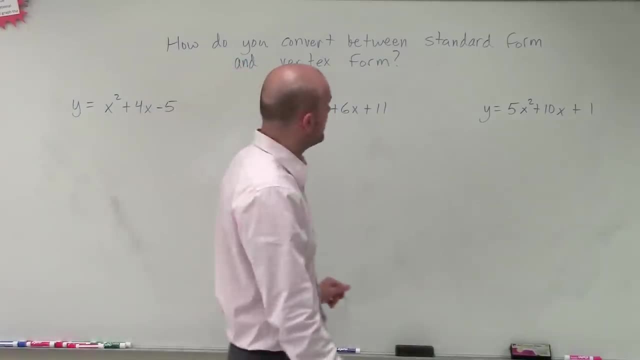 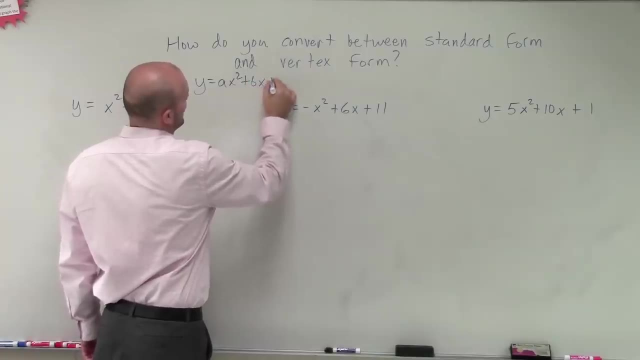 standard form to vertex form, So I figured I'd make a nice little video for you to do this. So what we're planning on doing is going from y equals ax squared plus bx plus c and converting that to y equals a times x minus h squared. 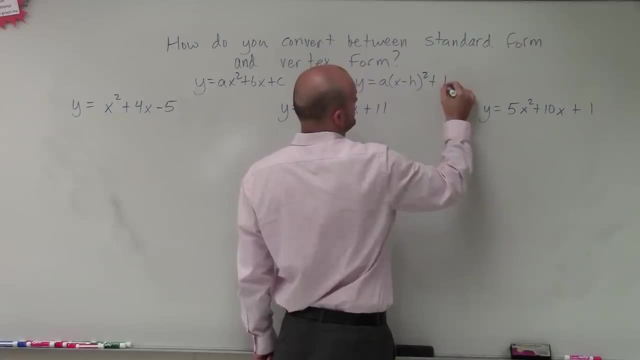 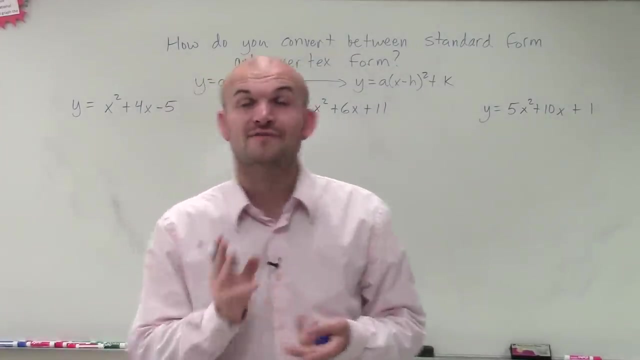 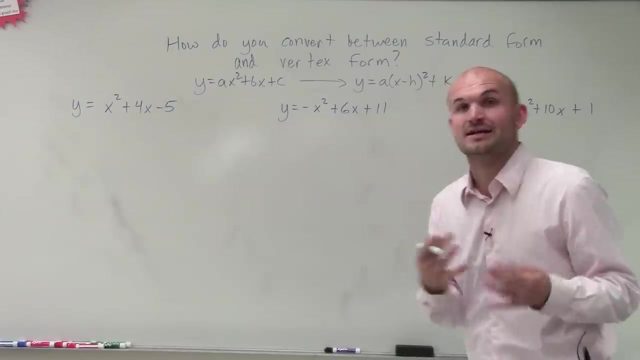 plus k, And you know there's a lot of reasons why we want to go through from standard form to vertex form. A lot of times it's easier to graph, it's very easy to find the vertex and so forth. However, it's not always so simple to convert from one to the other. So what I did is 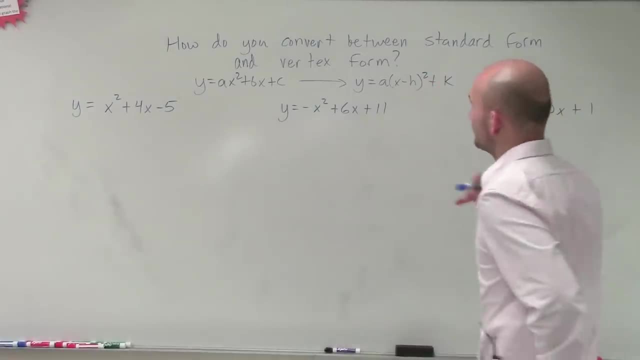 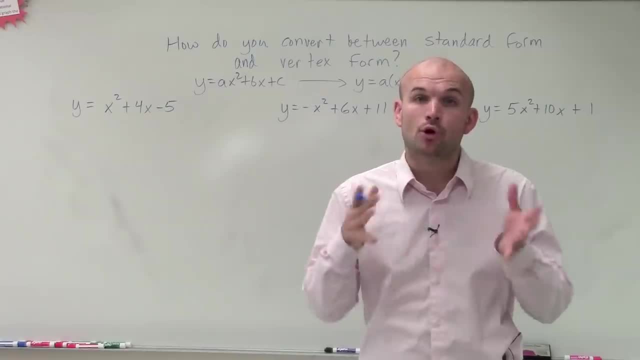 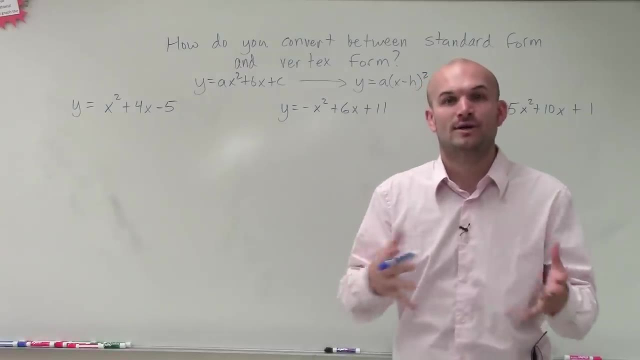 binomial and we square it. what we get is what we call a perfect square trinomial. All right, And that's what by what we're going to do is: we are going to create what we call a perfect square trinomial, And we're going to do that by what we call the process of completing the square. 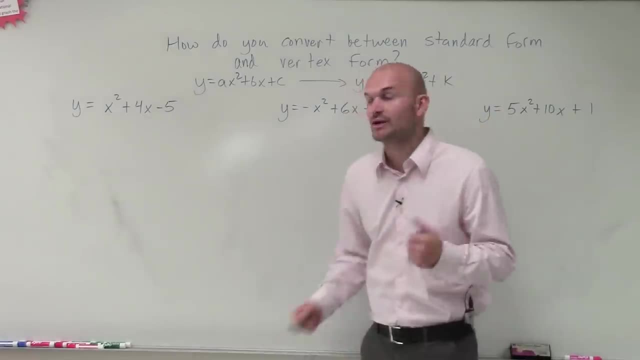 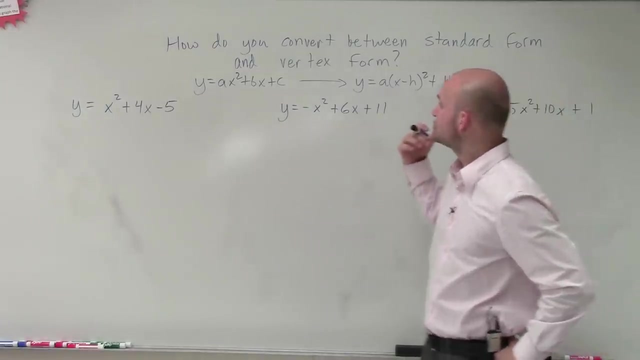 So there's going to be a couple steps, and I'm just going to kind of go through each one individually, And I'm actually going to do it for each problem all together. Now, the first step, though, we need to do is we need to make sure that, when we are creating a perfect